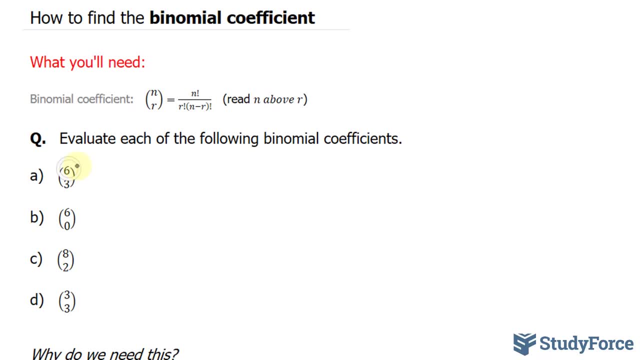 6 above 3.. So let's go ahead and substitute 6 where we have n in our formula, and 3 where we have r, We have 6, and this exclamation mark is factorial. I'll explain what that is in a moment. 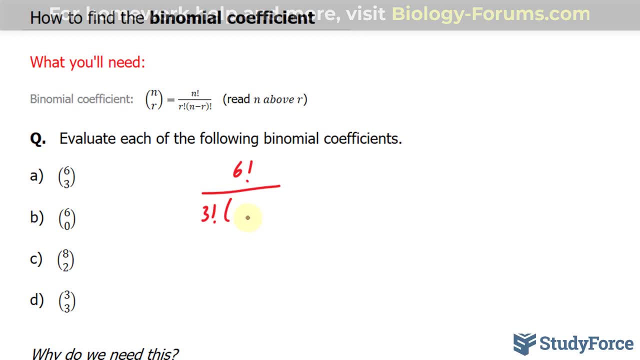 over 3 factorial bracket: 6 minus 3 factorial. I'll simplify this expression: 6 minus 3 is 3, so I'll replace this with 3, and now we have to determine what this factorial means. What this means is 6 times 5 times, 4 times, 3 times 2 times. 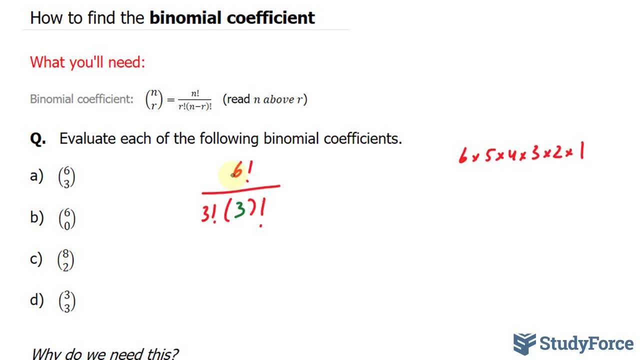 So if we have this expression at the top and 3 factorial at the bottom, which is 3 times 2 times 1, these factors will cancel out, leaving us with, at the top, 6 times 5 times 4 and at the bottom, 3 factorial, only this part: 3 times 2 times 1.. And if you put this into your calculator, you should: 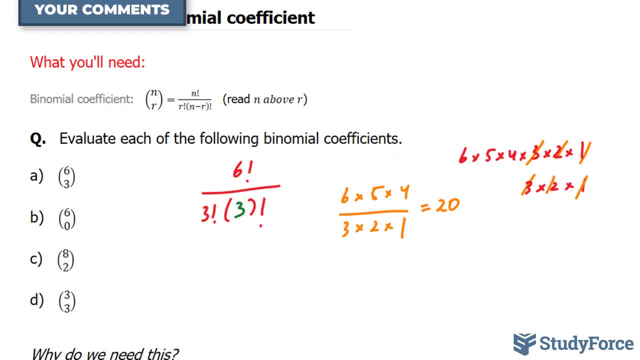 end up with 20.. Let's do the next one. This time we have 6 times 5 times 4 and at the bottom, 3 factorial, only this part, 3 times 2 times 1.. 6 above 0. So we'll write down 6 factorial over 0, factorial which is equal to 1 bracket 6 minus 0. 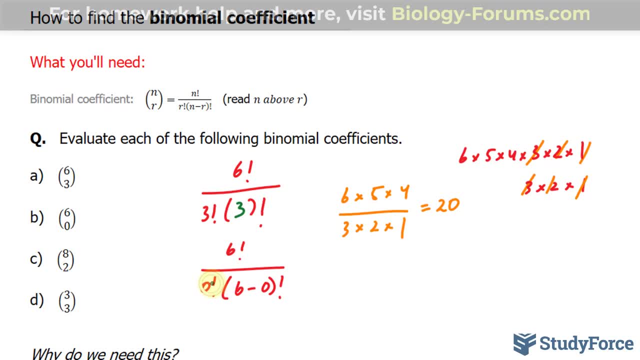 factorial. I just mentioned that this becomes a 1. We have 6 factorial at the top and 6 minus 0 factorial at the bottom. Therefore, our answer is 1, because we have the same factor at the top than we do in the denominator 8 above 2.. 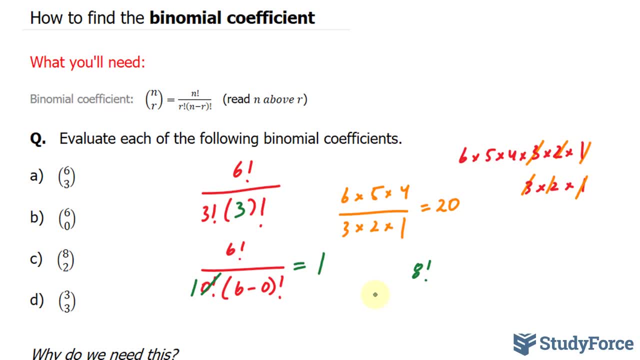 Let's go ahead and do our work over here: 8 factorial over 2 factorial. 8 minus 2 is 6 factorial. Let's go ahead and expand the numerator. We end up with 8 times 7 times 6, and I'll stop there. 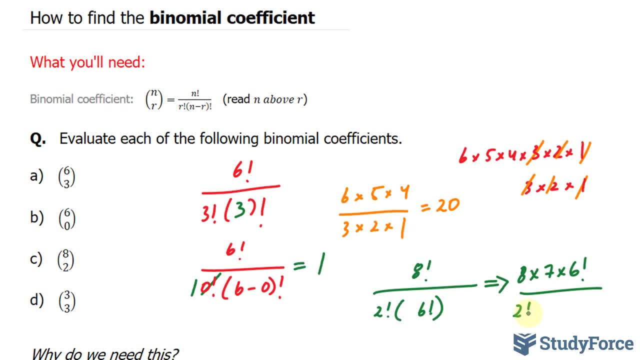 and write down 6 factorial at the bottom, This 6 factorial, and this will cancel out. So this cancels out. with this, We have 8 times 7, which is 56. Divided by 2 factorial, That's 2.. Our answer is: 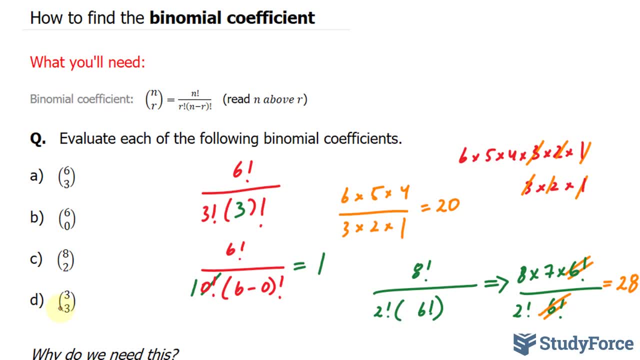 28.. Lastly, 3 above 3.. We'll work over here, since we're running out of room. 3 factorial over 3 factorial. 3 minus 3 is 0 factorial, That's 1.. We have 3 factorial and 3 factorial at the bottom. 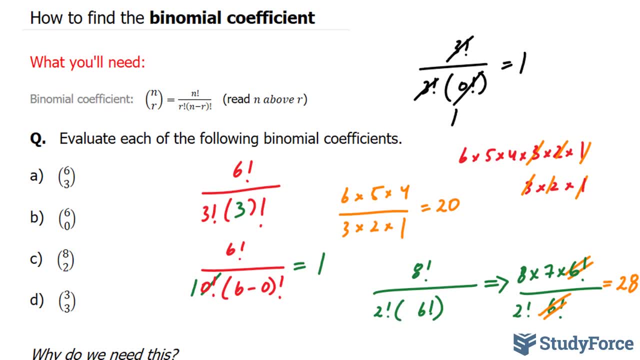 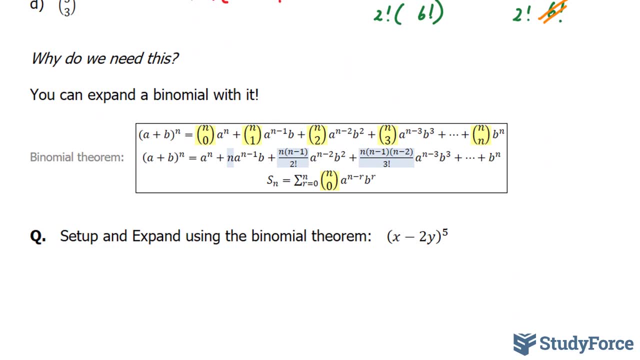 Those cancel out, leaving us with 1.. Now you're probably wondering why we even doing this. What's the point of the point of finding the binomial coefficient? Well, if you recall, we have looked at the binomial theorem in the past and the binomial theorem gives us a way to expand binomials. 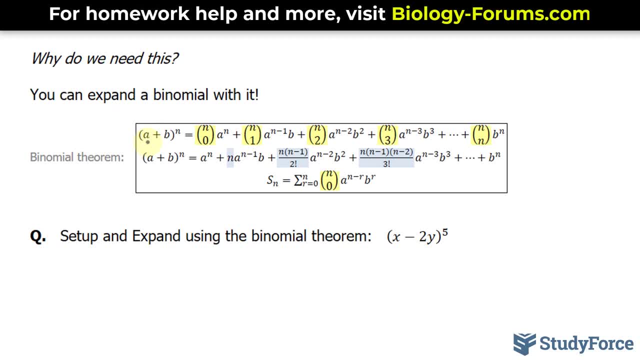 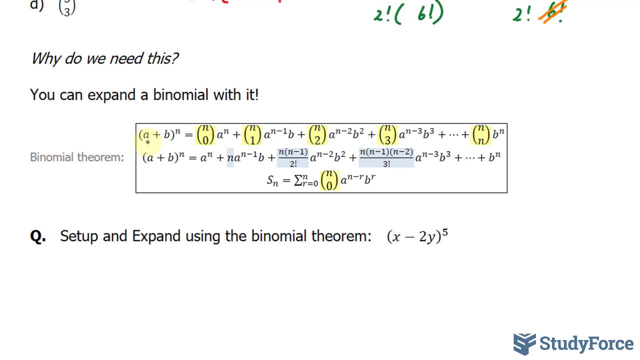 of nth exponent. So if we had a binomial, let's say a plus b to the power of 100, we can use the binomial theorem to help us expand it without having to do it manually. And what we were finding in question one were these things: what's highlighted. So let's go ahead. 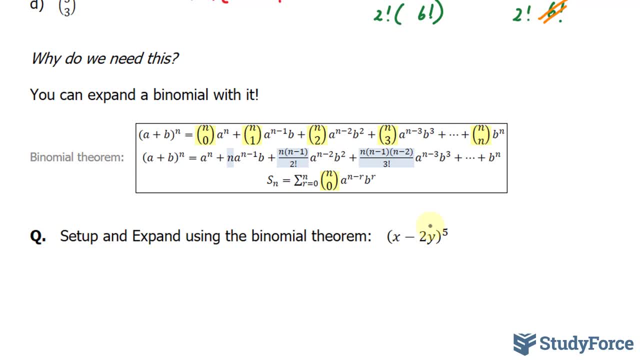 and set up and expand using the binomial theorem here, using the knowledge we just acquired in the first question. Here we have an, a value of x and a b value of negative 2y. Our n, which is the exponent, is 5.. So all we have to do is set up and expand. So the first 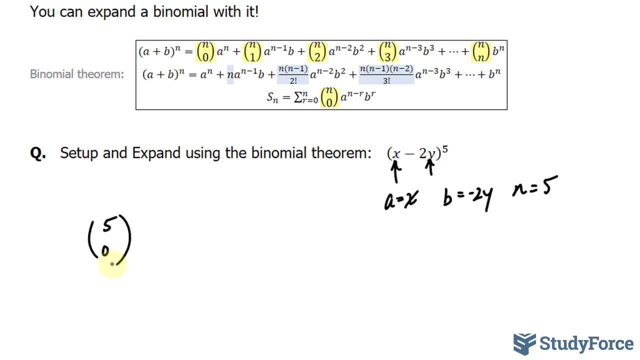 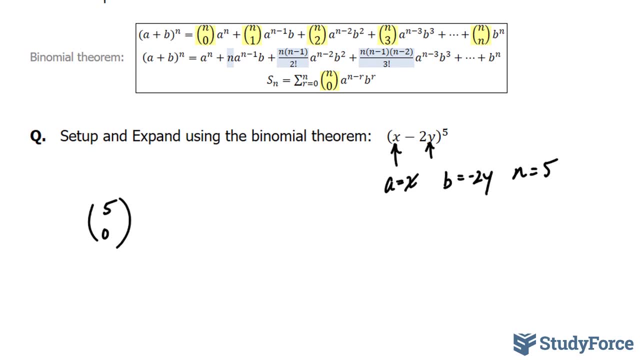 one will be 5 above 0. And we discovered that when it's a number above 0, the answer is 1.. So the first term will have a coefficient of 1, always. Hence we have a to the power of n, Our a. 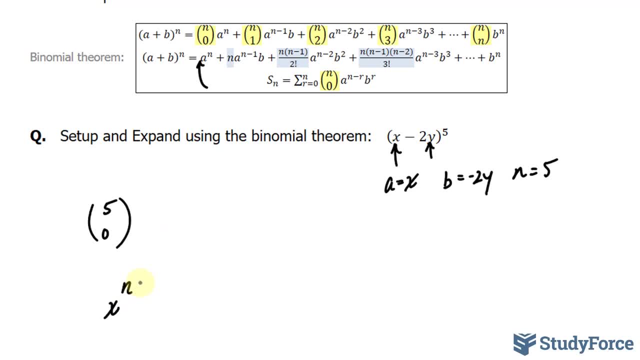 is x. x to the power of n is for the first one. And, of course, don't forget to substitute the n with a 5.. Then we have 5 above 1.. And 5 above 1 is the exact same number as the first one. So we have 5 above 1.. And 5 above 1 is the exact. 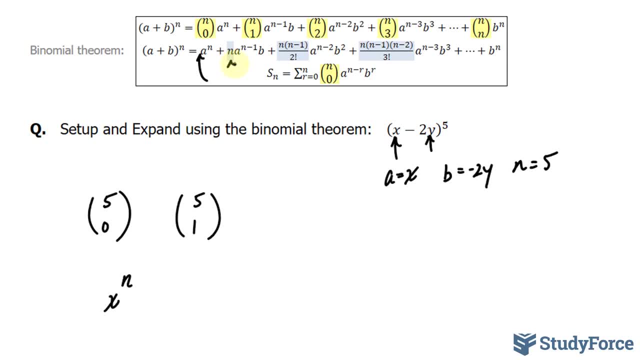 same thing as simply n, as highlighted in blue here. So we have x to the power of n plus our second term is 5.. a is x raised to the power of n minus 1, which is 4, times b negative 2y. We'll do one more term and then I'll show you the final expression Next.